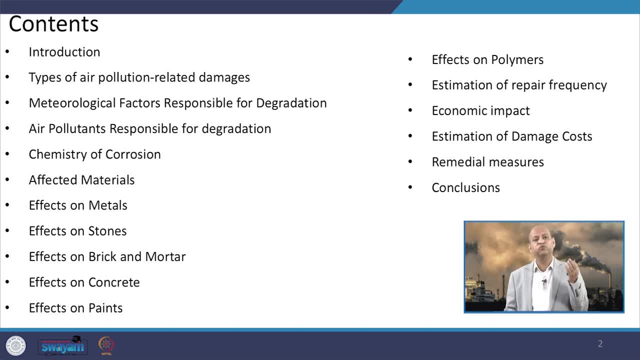 of air pollution, and then the air pollutants which are known for the degrading building material. then chemistry of corrosion, because the corrosion and abrasion, these two factors are very important when we talk about the relationship of air pollution or the weathering of building material. Then we will see the effect. 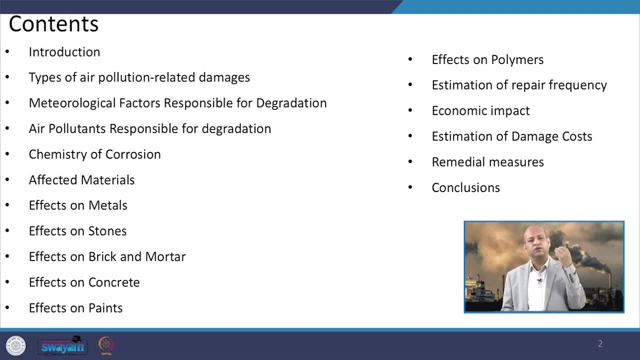 you know those materials which are affected, and on different kind of material, like on metals, stones, what kind of effects are there? We will also see on the brick and mortar effects of air pollution and then the on concrete, paints, polymers, etc. 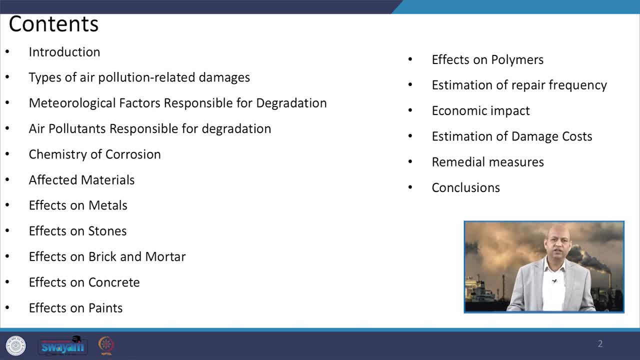 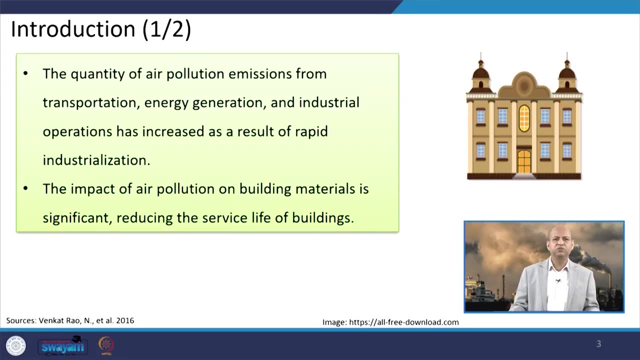 Then we will see how, you know, repair frequency is, you know, estimated by that particular range of the cost parameters and the economic impact and the estimation of damage cost and then the remedial measures and we will conclude accordingly. So when we talk about, you know the air. 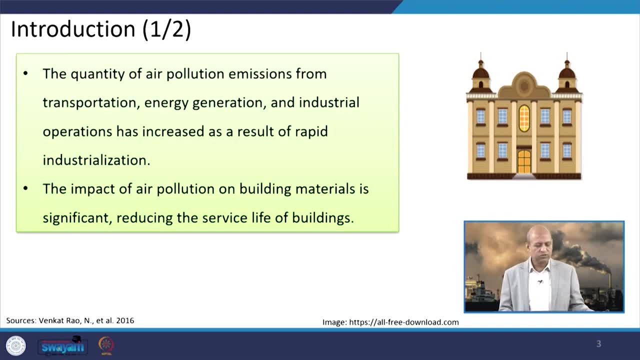 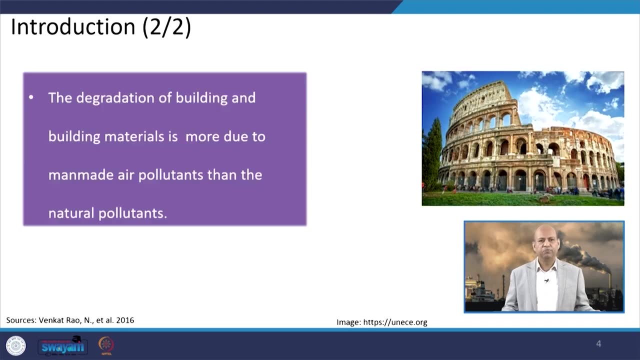 pollution relationship with the buildings. so, basically, you know, all kind of air pollutants have certain effects on the buildings and it can, you know, affect the buildings appearance as well, as it can also damage the structural component of the building. So it can reduce the life of the building and it is also, you know, found out that 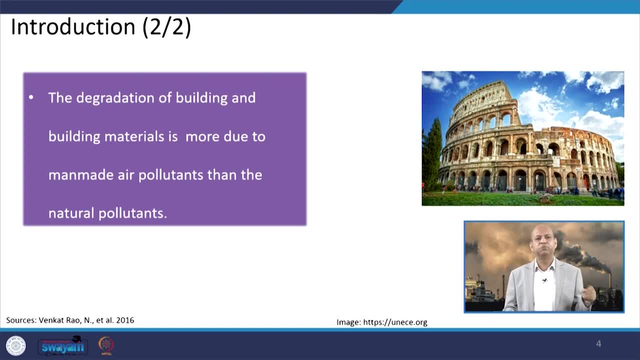 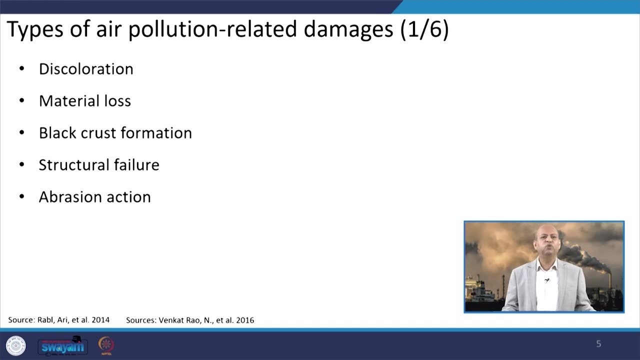 the air pollutants which are emitted by manmade activities. they are more responsible in comparison to the natural pollutants to damage the buildings. So we will see accordingly those aspects. Well, when we talk about types of air pollution related damages, so those can be classified. 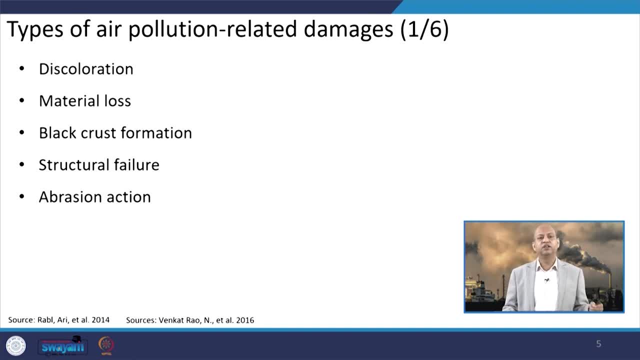 like it can discolor the building or it can have result in losses of the material. Then it can also cause like black-colored às the layer of floor material. so thatï is said to be less war. Well, when we talk about types of air pollution related damages, so those can be classified like it can discolor the building or it can result in losses of the material. Then it can also cause like black-colored and you know it is. it is lot of loss early Now. there can be there a loss in material to the opposite of that which taken the material and it can also caus kerupal touring houses. 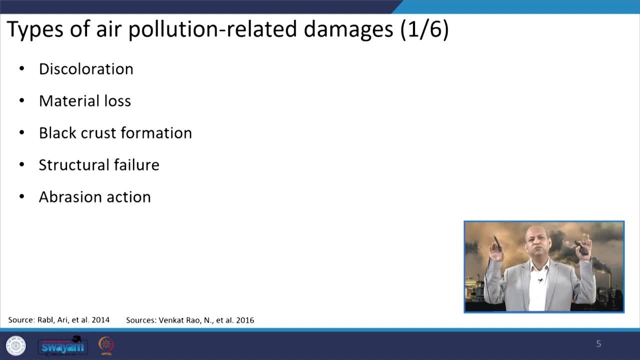 and therefore it related to spillage systems etc. that such as what we see common, which colored crust formation, you might have seen discolored buildings, even if they are painted. so after one season, like monsoon, you will see blackish or grayish or sometimes greenish kind of. 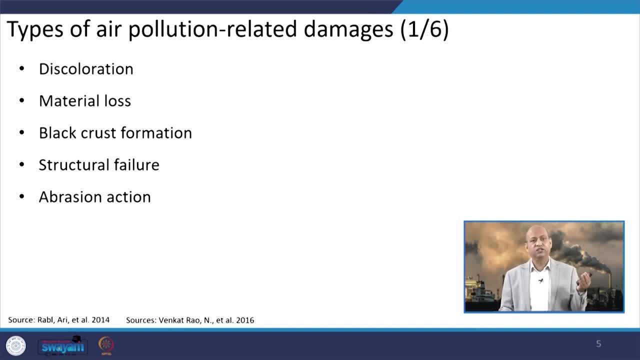 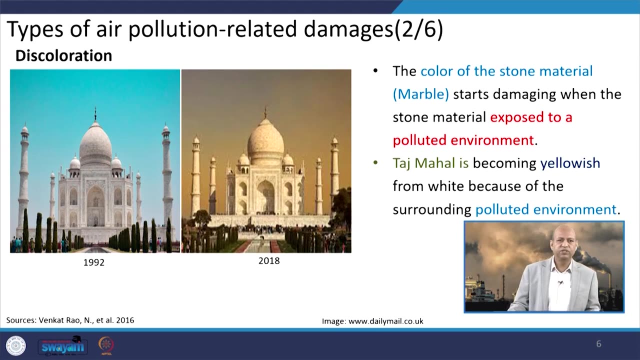 color is there, then structural failure may be there because of long term effect of these air pollutants and abrasion action, because when friction is there and particulate matters etc. the constant abrasion happens. then the building is damaged. So you can see the effect from pictorial representation. like you know about the Taj, 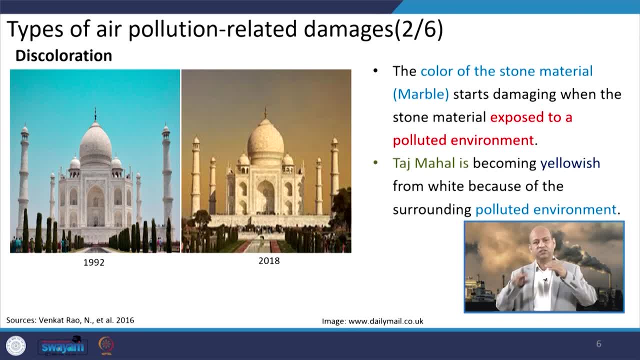 Mahal. it is said that because of pollutants, the appearance of the Taj Mahal stone, this marble, from white it has been to yellowish. so that has been because of particulate matter as well as the sulfur dioxide related or other kind of pollutants which are present in the. 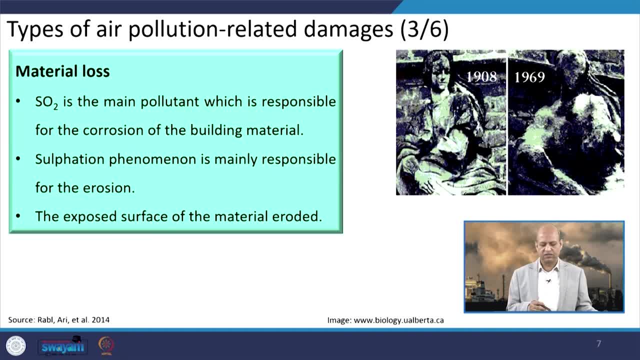 air When we see these kind of structures, artifacts. so in 1908, all you could see those features of this particular statue, but in 1969, over the years of around 60 years or 61 years, all those features has gone and the reason is because this acidic rain, or this acid rain as 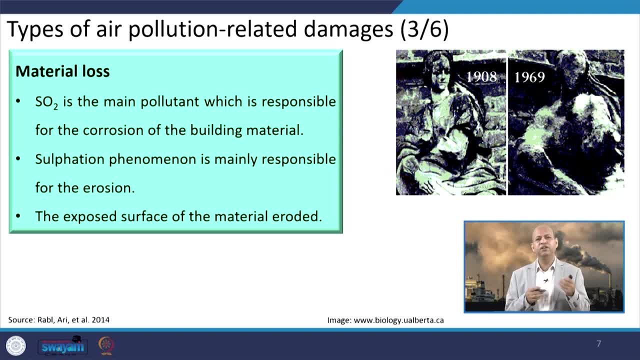 well as the abrasion because of particulate matter. all in combined, you know weathering effects etc. they result into such kind of damage to very important artifacts of our history. Well, it is also known that in stone materials they have like porosity, as you know. 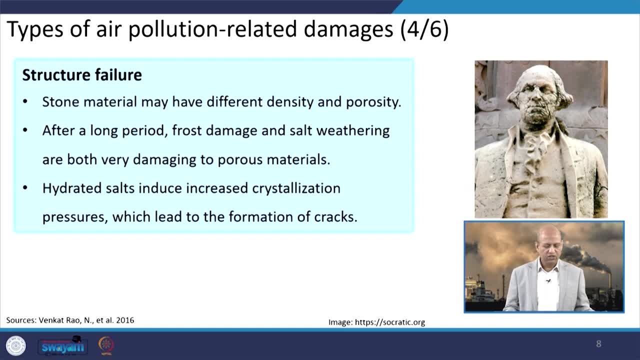 and different densities at different places. So accordingly, after a long period, like frost happens, so because of temperature increase, then temperature decrease, so this weathering effect happens and this porous material is more susceptible for for those kind of things. And then the hydrated salts which go inside. you know, these pores and 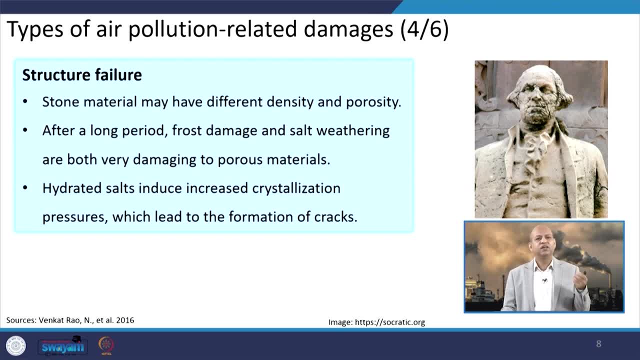 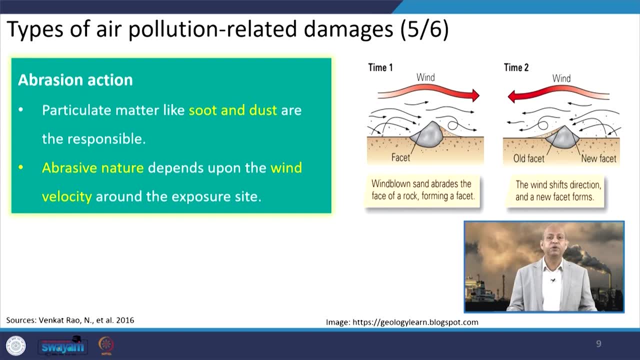 they crystallize and they generate the pressure and that can lead to some cracks etc. from inside to outside. So you can see this effect of you know this abrasion action. So if you know, that kind of feature is there, so wind is coming, particulate matters are also there and because of that, 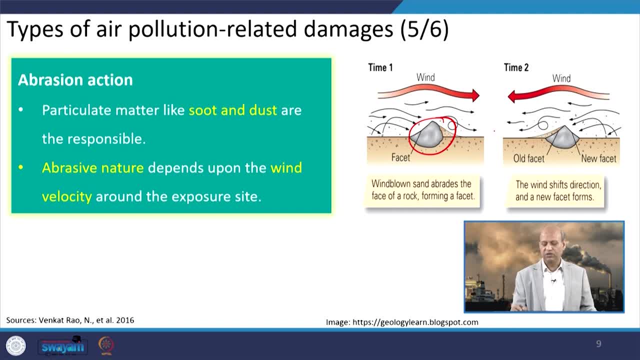 you know this kind of situation occurs and according, you know this kind of- you know- dust deposition happens. So over the period of time, their surface get abraded and it gets damaged. You can see the old facet and the new. 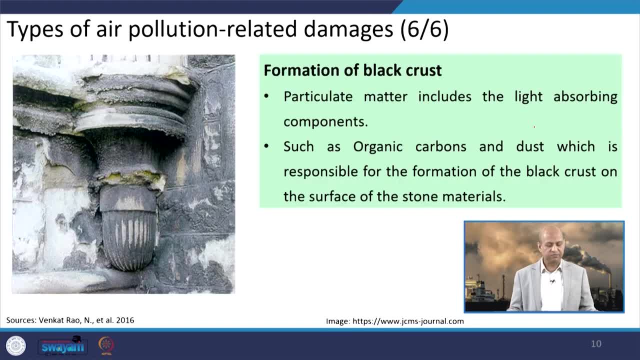 facet because of changes due to the abrasion. And then we talk about this black crust formation. you see, these kind of. you know, deposition occurs because of particulate matters, which absorbs the light and black carbon, organic carbon or dust moisture, everything you know. 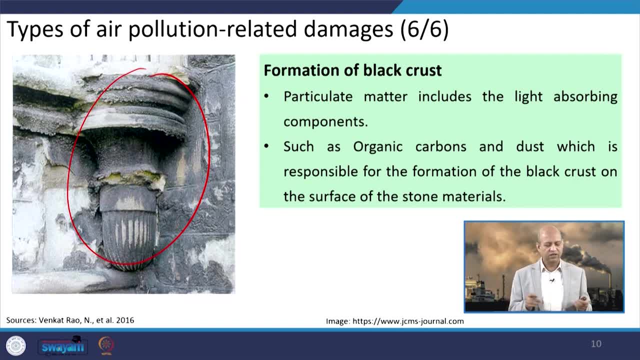 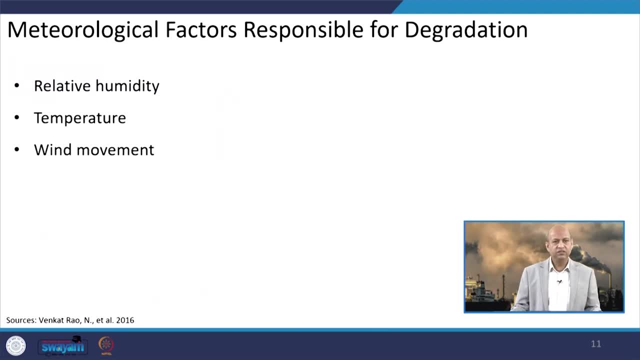 mix and then they get deposited on certain places and they disfigure as well as they also cause chemical and physical damage to the property. Then there are, you know, meteorological factors, which enhances these air pollution related damages to the building material and buildings. 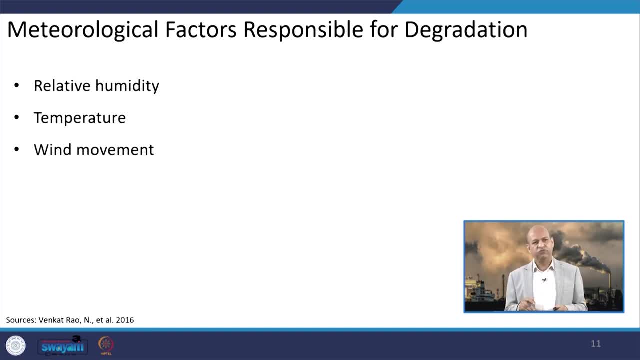 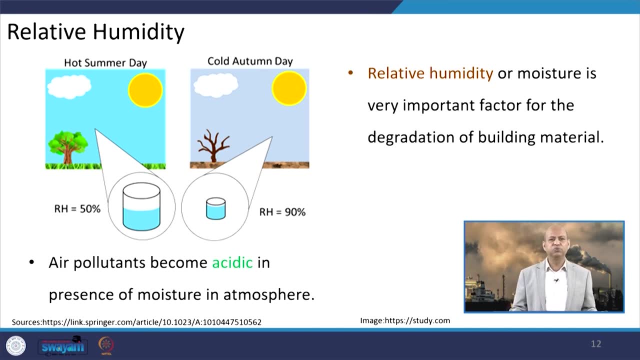 So these are like relative humidity, temperature, wind, movement, and we will see how they affect. like when we talk about relative humidity, they basically, you know, contribute into acid drain because they react with sulphur dioxide or nitrogen dioxide and in that way they can cause. 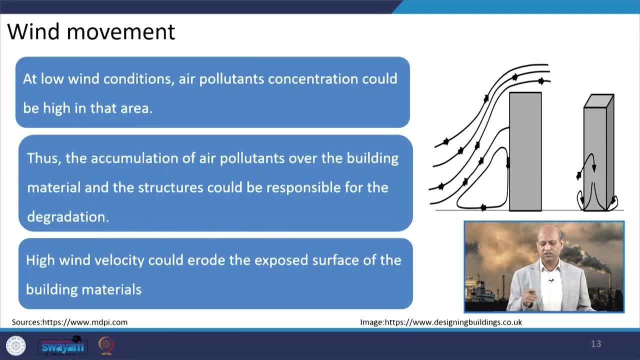 the damage to the building material. Wind movement has its own effect because of certain patterns, So they are responsible for deposition of particulate matter. they take the particulate matter along with them. then abrasion occurs, friction occurs, they damage the surface. 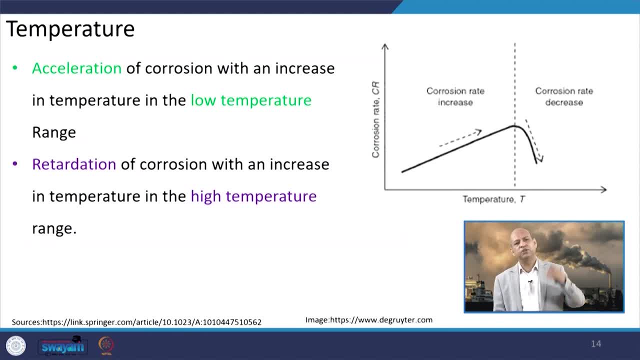 the building Temperature, basically temperature difference in different kind of materials. they get expansion, then contraction, so that changes its physical phenomena and it causes the damage. but high temperature, this corrosion related effect does not occur because moisture is not there. otherwise corrosion rate increases with the temperature. this is the result of a study. 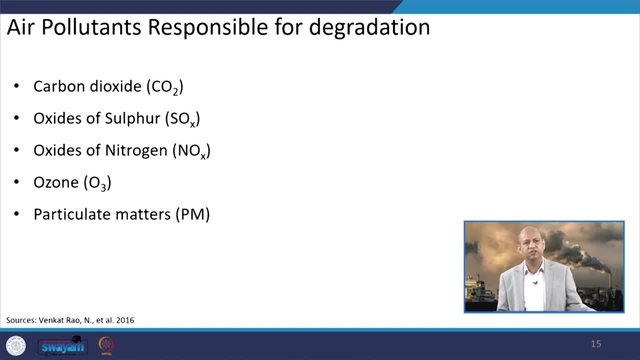 When we talk about air pollutants which are responsible for degradation. so the major air pollutants which are responsible for degradation of buildings are basically carbon dioxide, oxides of sulphur, oxides of nitrogen, ozone and particulate matter. Now you can see the difference. health effects may be there, like VOCs and other pollutants are there. 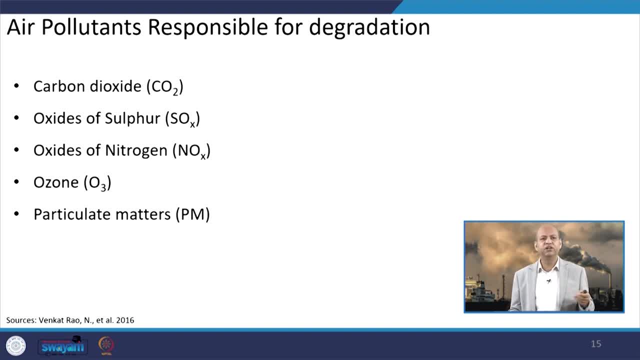 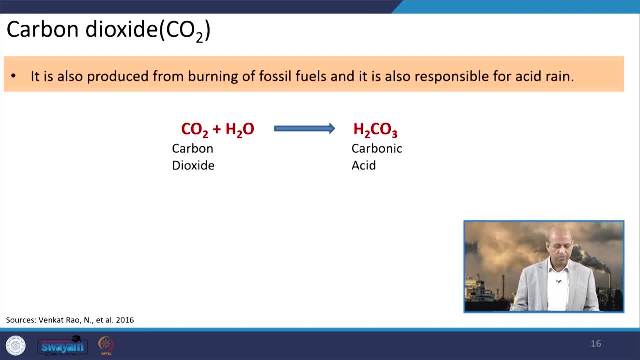 they are responsible for health effects. but when we talk about the building damages, then only a few are listed here which are majorly contribution of air pollutants. Well, when we see this carbon dioxide, because of moisture in the air, this carbon dioxide gives this formation of carbonic acid and that is why the rain water always has somewhat lower pH. 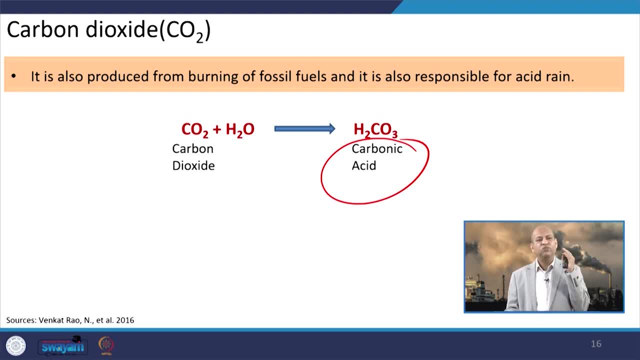 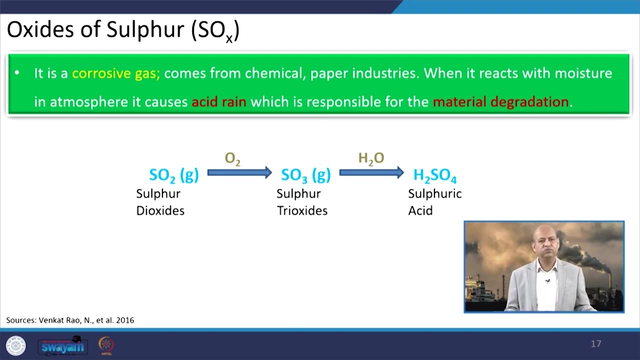 but we do not call it acid rain. acid rain is called only when the pH is very, very low of the water. So this is always present in the air and this causes this acidic kind of behaviour of the air, moisture and the oxides of sulphur, as we have seen. 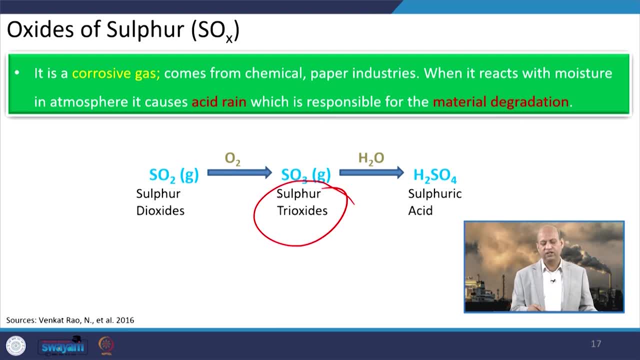 that it can get converted to sulphur trioxide. then, because of moisture, it can convert it into sulphuric acid and sulphuric acid is very, very corrosive, as you know, and that is why the SO2 high concentration in air is the major cause for damaging the building materials. 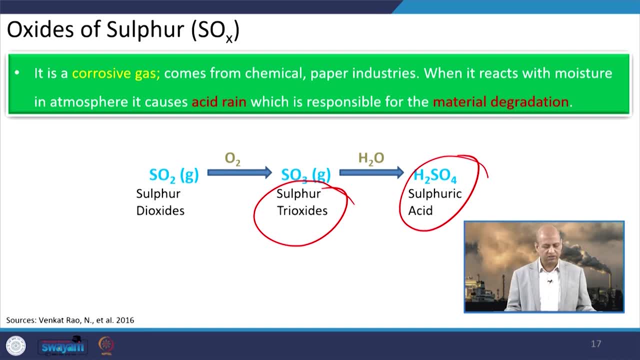 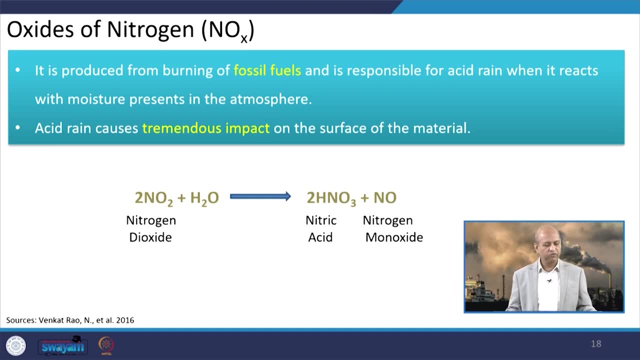 especially like calcium carbonate related building stones And metals like iron, ferrous related. we will see that in detail When we talk about oxides of nitrogen. so again, because of moisture it is converted to nitric acid, but it is not as much damaging as sulphuric acid. but it is also the cause factor for the acid rain. 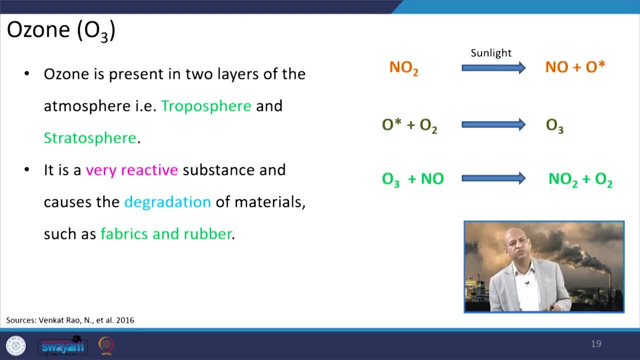 Ozone. as you know, ozone is a secondary pollutant formation in the troposphere because of photochemical reactions, like in the presence of sunlight. NO2, it goes to No and O and then one molecule of oxygen. when it is connected to this atom, then 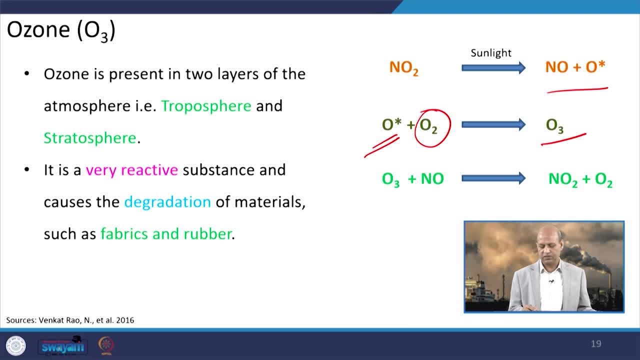 ozone becomes in existence and this is a kind of titration reaction. So No, if is there from like transport sector-vehicular emissions, it can give a NO2, so that is why this is the titration effect, that in city centres, where lot of emissions are there- from vehicle exhaust emissions- 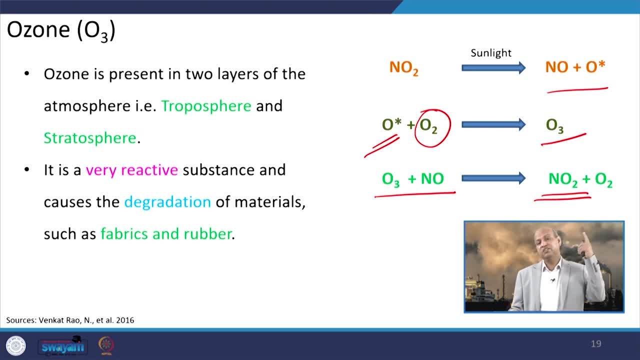 emissions, so ozone is less there, but in countryside ozone is more because this NO2 goes with the downwind pattern in the countryside and sunlight is there and this gives the formation of ozone, So that cyclic reaction occurs all the time and ozone is very reactive as it is very highly. 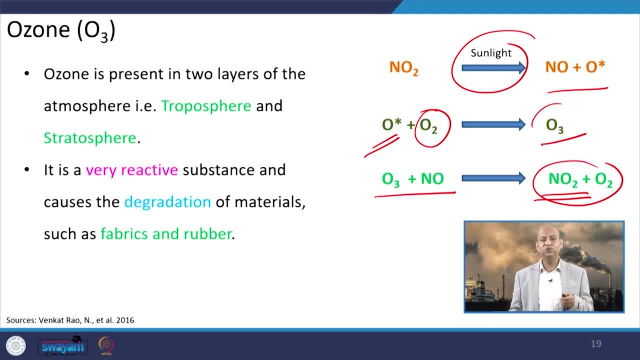 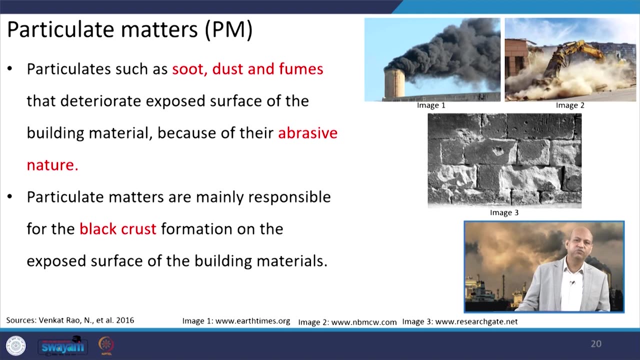 oxidizing gas and it is also greenhouse gas. This is also interesting to see. ozone is not only the health damaging pollutant, but it also contributes to global warming and climate change related issues. Particulate matter when we talk. as I said this particulate matter in the last lecture, as 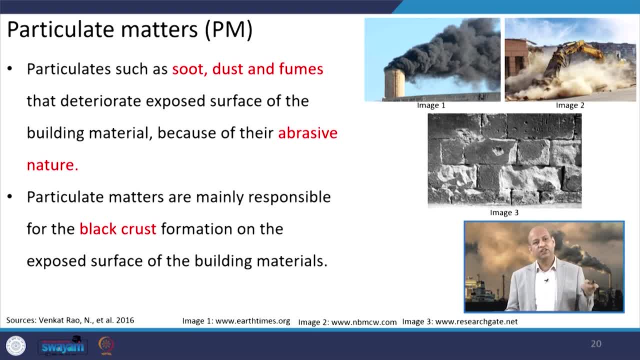 I said that it caused several kind of health effects and it is also responsible for several kind of building degradation. You can see the sources of particulate matters, which occurs in terms of soots, smokes, and then these activities, construction activities. so they have this abrasive in nature because friction occurs whenever they strike to the 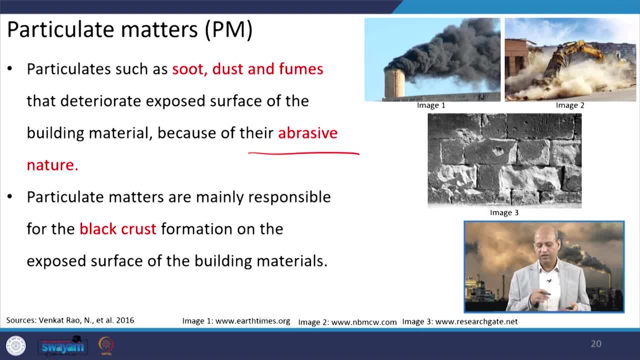 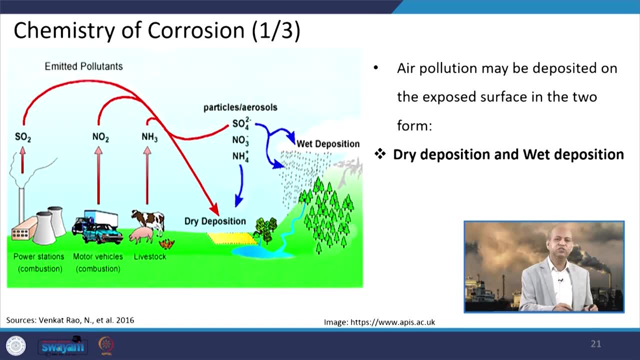 surface, dry deposition can occur and then it can slowly damage the surface of the building. When we talk about the chemistry of the corrosion, basically so the emissions of sulfur dioxide or nitrogen dioxide, ammonia, etc. they go into the air and then dry deposition occurs. 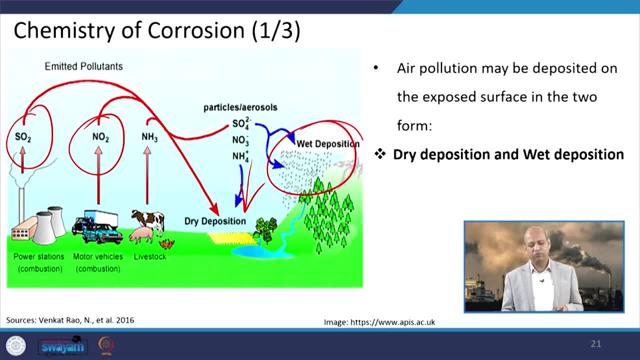 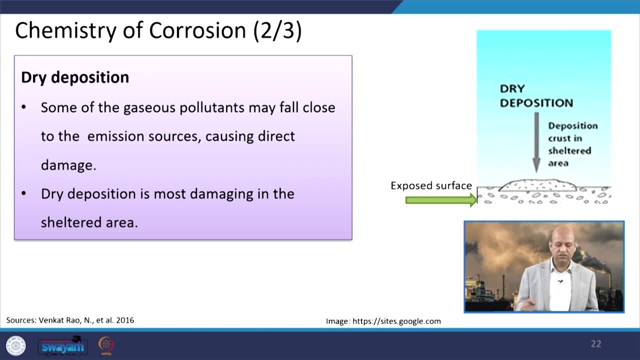 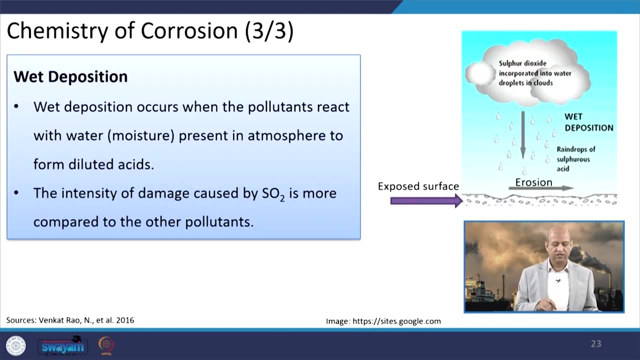 wet deposition occurs. so then this acid rain, basically formation, is there and this acidic effect is there. So the corrosion effect is, because of those reasons, Dry deposition, simply because of gravity, particulate matter, even gases that descends to the surface, and the wet deposition because of that precipitation effect is there and that 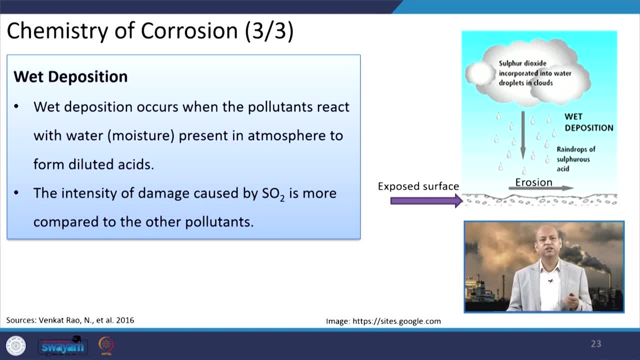 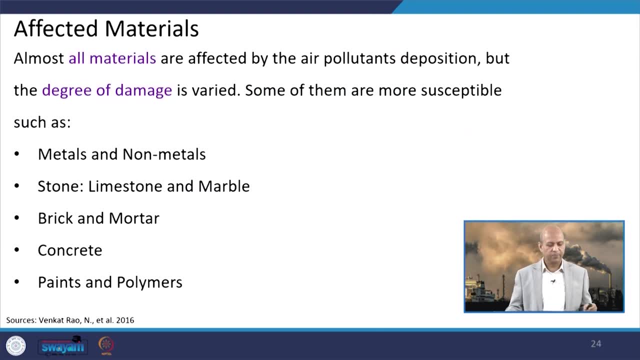 is more dangerous for building material etc. if there is lot of SO2 concentration in the air and that is got converted into sulfuric acid. So when we talk about how material is affected, so we can see all kinds of materials are affected by these air pollutants. 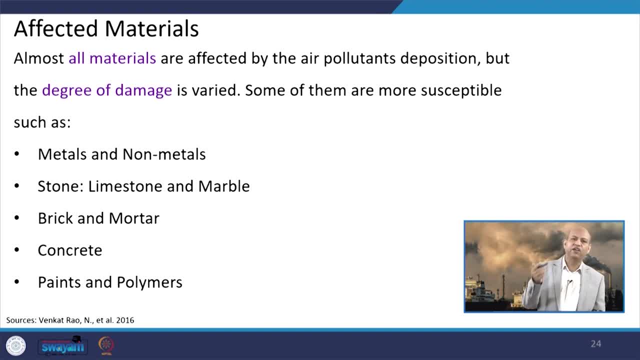 whether they are metals or non-metals, even stones like limestone or marble, then brick and mortar, concrete, paints and polymers- all these building materials are damaged in one or other way by air pollutants, and we will see how they are damaged. 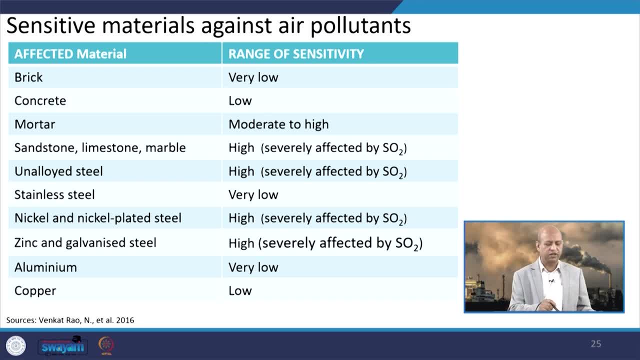 So you can see the sensitive materials against air pollutants, like brick. it is not so much sensitive to the air pollutants because of its at high temperature it is manufactured and it is not so much susceptible. it can afford to be exposed by high concentration of those kinds of air pollutants. 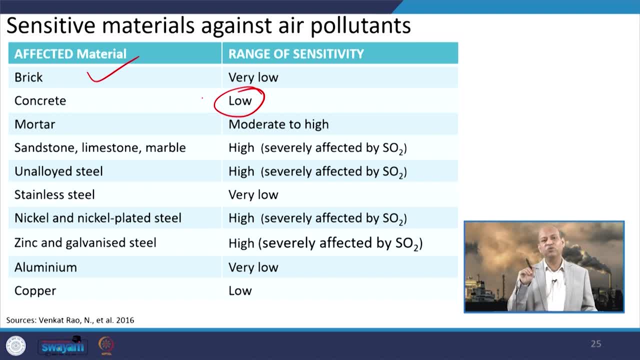 Concrete is also low. but once concrete is damaged and somehow this acidic water goes inside and if it starts corrosion of the reinforced that, the steel or iron, that ferrous material, so because of rust the volume increases and then concrete starts to crack and then this can get affected. 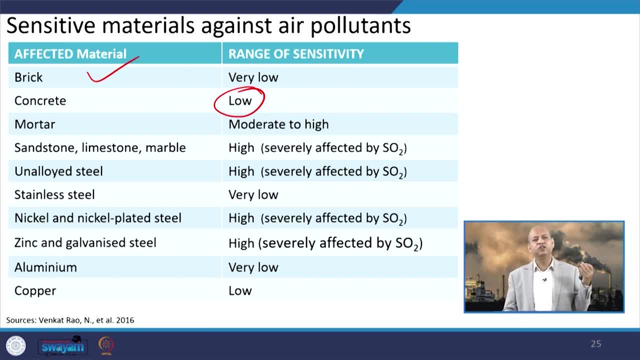 But if also you can have very high grade concrete which may not be affected but that is very expensive. Mortar, moderate to high effect may be there because of air pollutants: Sand stones, limestones. they are high because of this SO2.. Similarly, 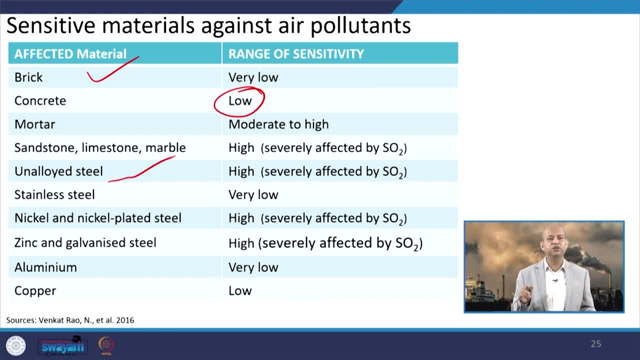 this unalloyed steel is also highly susceptible to air pollutant because of SO2.. Stainless steel, as you know, because stainless its name is there, so that is very low affected by these acidic pollutants- Nickel plated steel, etc. they are again because of SO2, zinc galvanized steel. 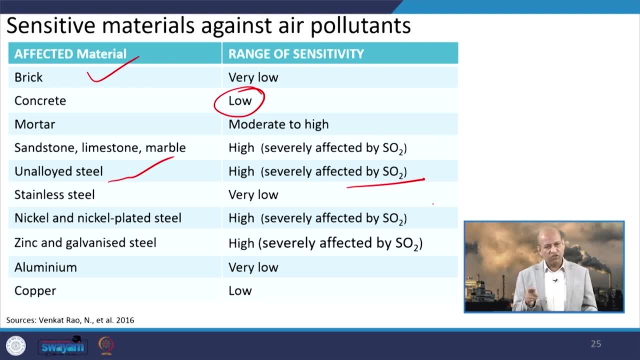 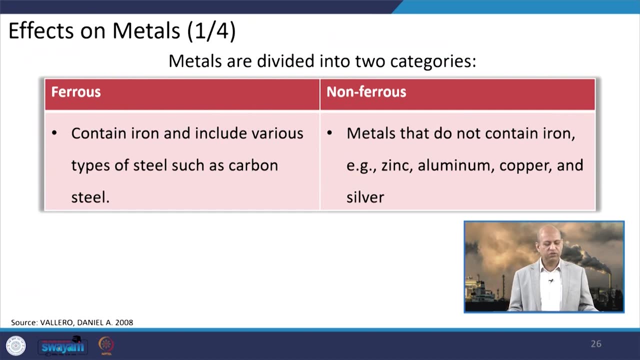 all these are highly susceptible. Then aluminum, very low, but aluminum has its own problem, you can know about that, but at least from this air pollutant it is not so much problematic. Copper has low, but it is affected When we talk about these metals, so ferrous metals, they are affected by severely by SO2,. 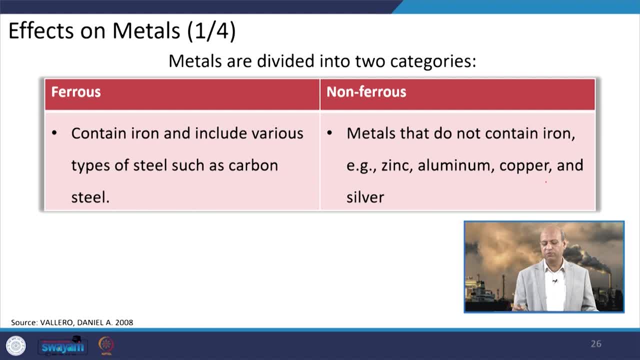 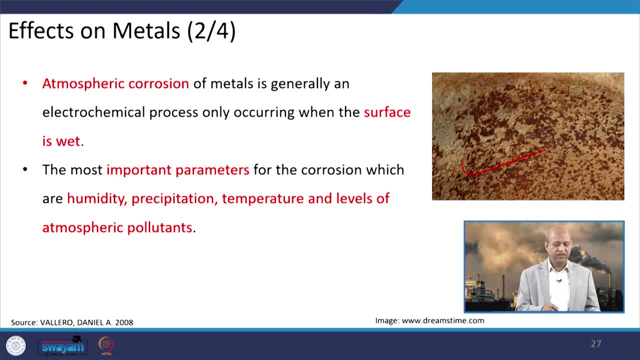 etc. non-ferrous, like zinc, aluminum, copper, they are not so much affected And, like you can see this figure, this corrosion effect is there and this is because of this electrochemical process which occurs in the wet surfaces, because of these air pollutants. 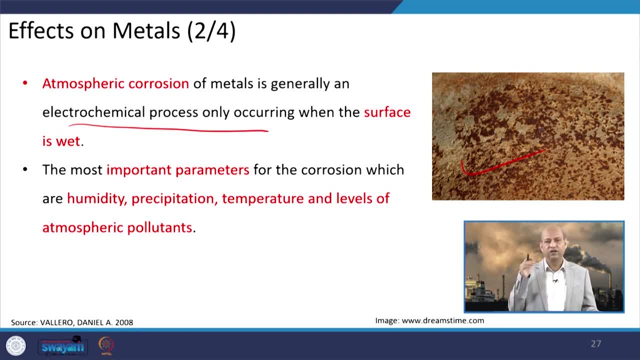 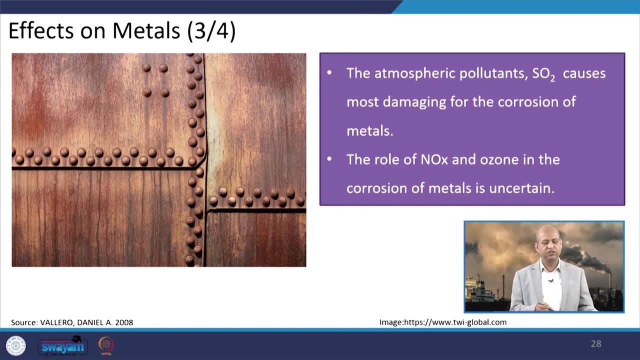 And the important parameters which affect the corrosion reactions are like humidity, humidity, precipitation, temperature, levels of atmospheric pollutants. all these will govern how much corrosion may occur and how much it may be damaged. You can see, these kind of iron gates can be affected by corrosion and rust because of these SO2,, etc. and NOx also has some effect. 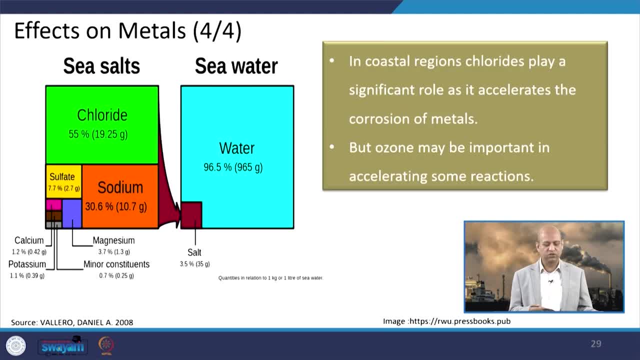 ozone corrosion on the metals is uncertain means more research is needed. When we talk about at the places like seashore, so, for example, you can see this lot of salt and with air, salt comes to the air and within salt. 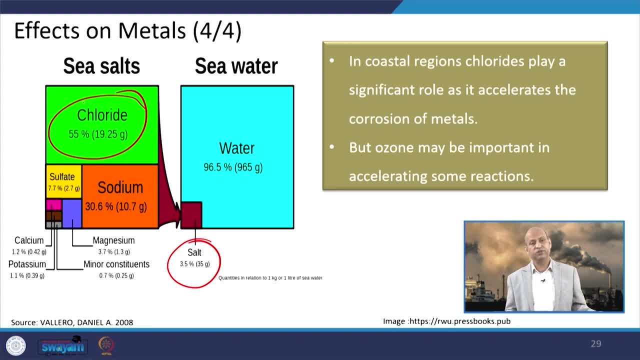 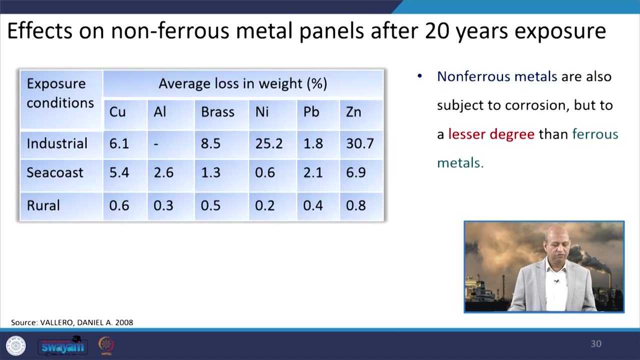 if you see, like sulphate sodium is there but the huge quantity portion- 55 percent, more than 55 percent- is chloride and that plays significant role when this corrosion related action is accelerated because of these chlorides. But ozone may be important in accelerating some. 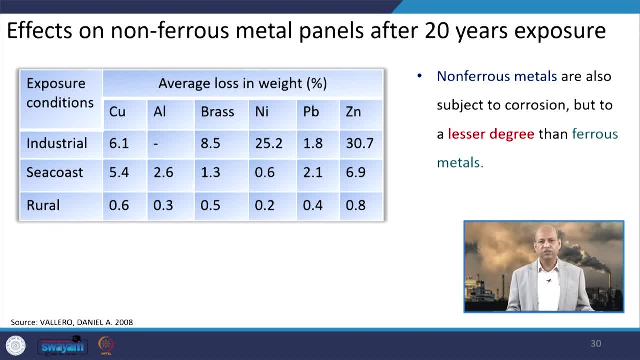 other reactions When we talk about effects on non-ferrous metals. so we can say that in the case of the sea coast, the exposure is very high. the exposure is very high. about 20 years exposure study has been conducted so you can see like: 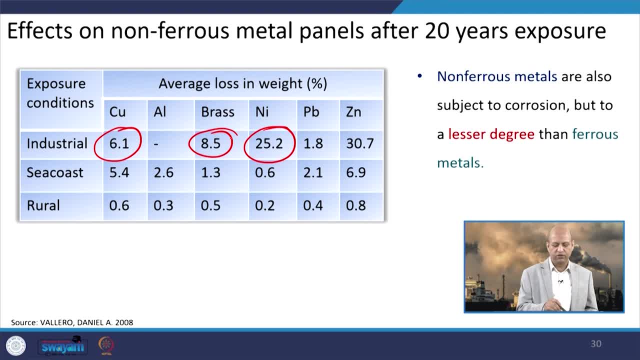 exposure conditions. in industries it is very high: 6.1, on the, brass 8.5,, nickel 25.2.. In sea coast it is less than the industrial area. In rural it is further less. So you can say that. 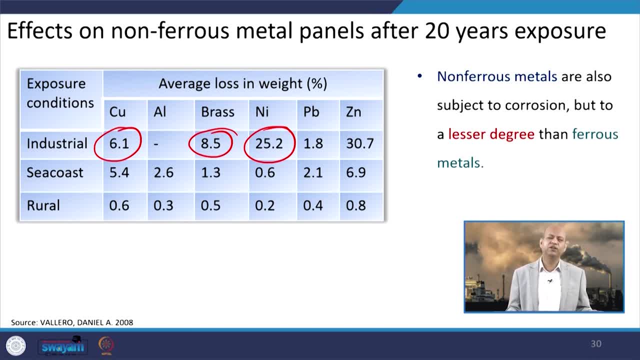 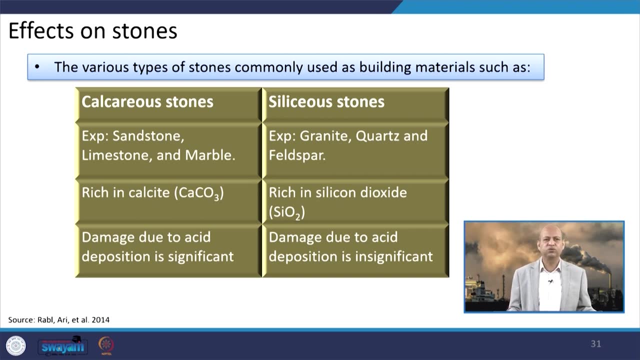 industrial because in industrial areas lot of pollution is there and the air is polluted in terms of sulphur oxides or particulate matters or other kinds of toxic materials are there When we talk about the stones, effects on the stones because of air pollutants. 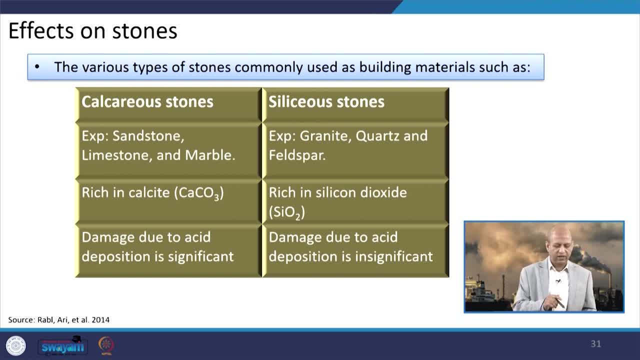 then majorly we talk about like calcareous stones and siliceous stones. So siliceous stones are more sturdy, like granite etc. They are very tough and they are not so much affected by these air pollutants but the sand stones, lime stones, marbles etc. they are very much susceptible to. 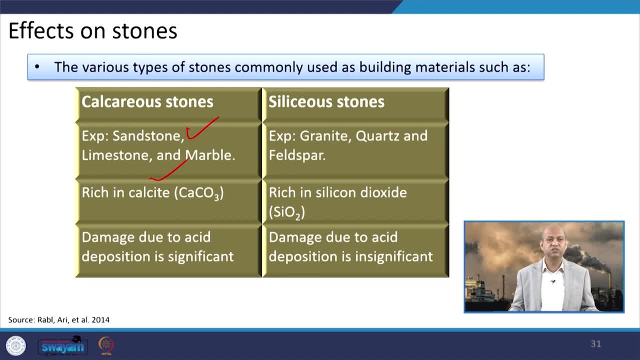 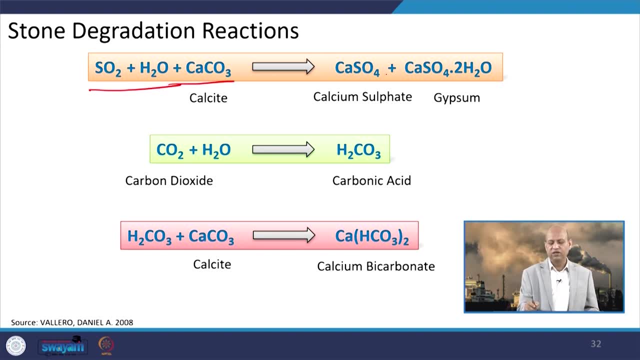 the SO2 pollutants because of this acid drain or acid deposition, They can be…. there is a very simple reaction, as you know, because CaCO3, SO2, S2 is there, So the calcium sulfate is formed, gypsum is also formed and this carbonic acid can. 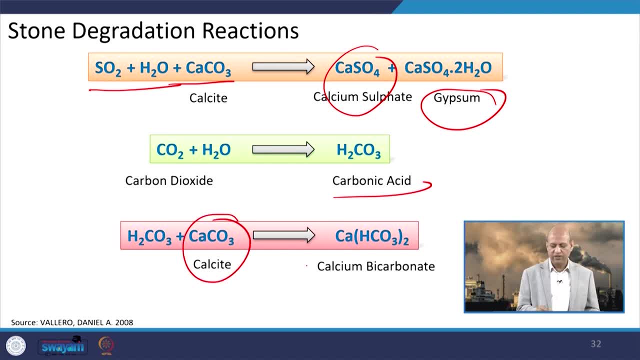 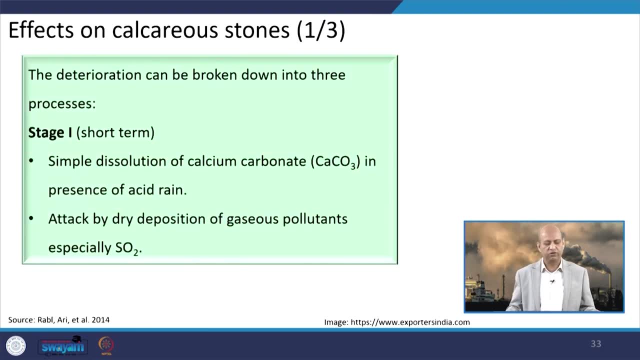 also participate to the CaCO3 and it is calcium bicarbonate is formed. So that kind of stone is of stone is very much susceptible to acidic atmospheric environment. When we talk about in continuation to these carious stones, then there are different stages. 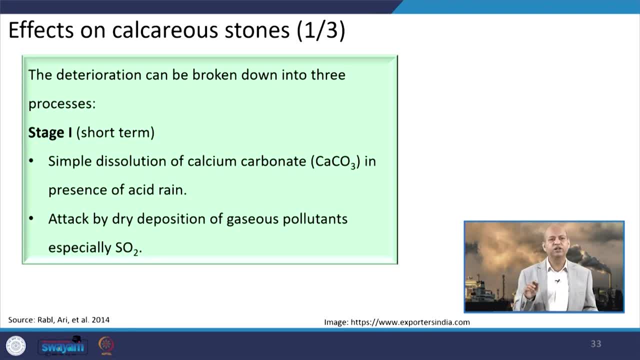 Like in stage 1, simple dissolution of calcium carbonate happens in presence of acid rain And the attack by dry deposition of gaseous pollutants, especially SO2, also occurs. But that is slow process. Then the stage 2, that is the medium term. 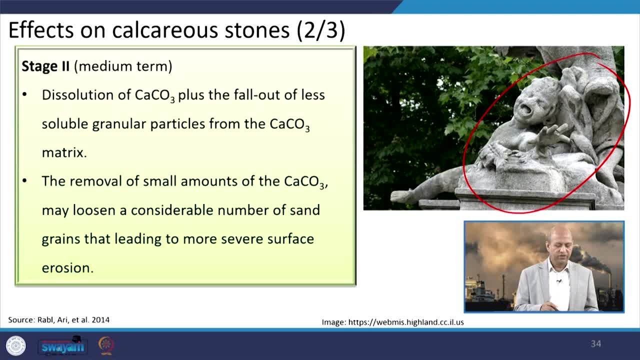 And you can see this is the effect of the second stage. So in this dissolution of calcium carbonate happens fallout and because of this acid rain the surface get damaged. because the dissolution has happened, calcium carbonate has gone to different kind of products like calcium sulphate etc. 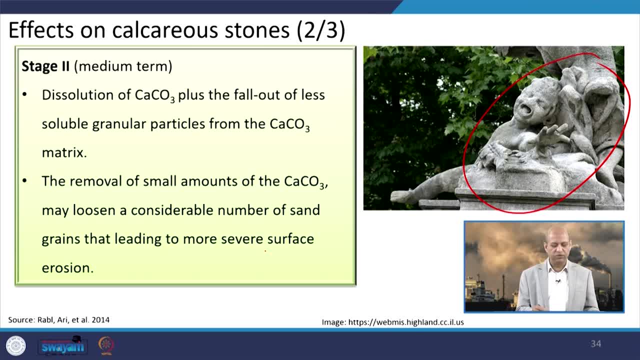 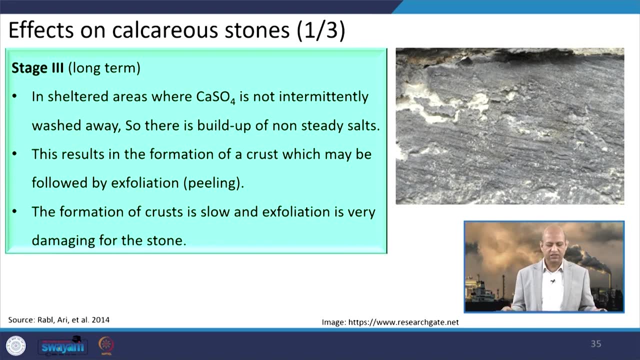 And the removal of a small amount of calcium carbonate may lose considerable number of sand grains And the leading to surface erosion And further. this acceleration happens because then more porosity is there and then more attack will be there because of acid rain. When we talk about stage 3, then in stage 3, basically this sheltered areas where calcium 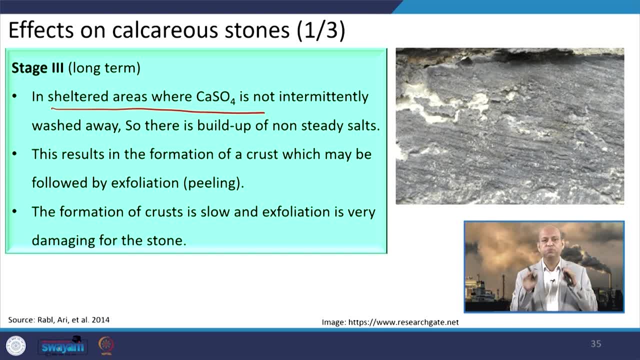 sulphate is not intermittently washed away. this is deposited there, So it can build up into the concentration and it remains there And this results in formation of Crust which may be like, followed by the peeling of that surface and the formation. 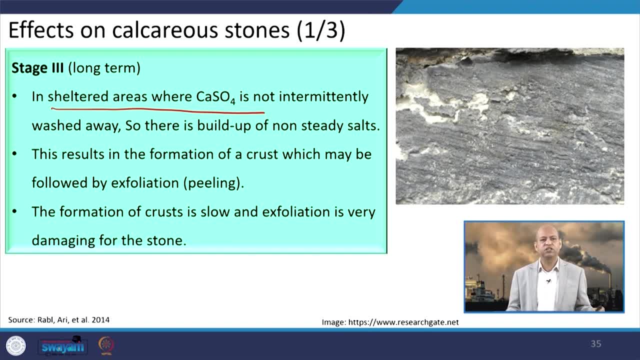 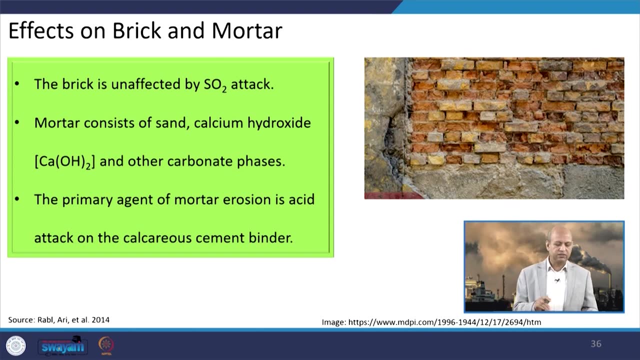 of crust in slow and this particular pulling process happens, the further damaging of stones happens. you can see here. So those kinds of things may happen. So three stages are there in calcareous stone damage because of air pollutants. When we talk about brick and mortar, the mortar again has certain calcium carbonate related. 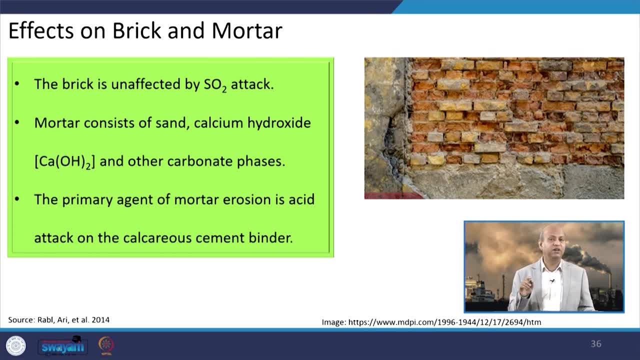 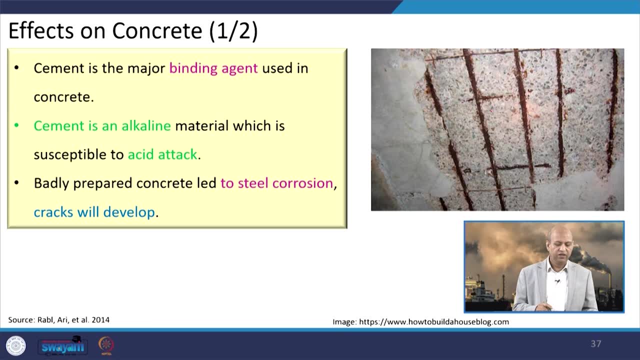 things. So that is affected. But brick is not so much affected by that. It is affected by SO2 attacks. So you can see the mortar. only those gaps are because of this acid rain. you can see When we talk about the concrete. so in concrete, basically, this reinforced concrete basically. 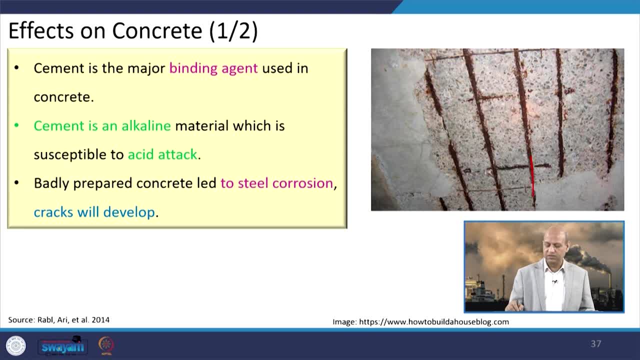 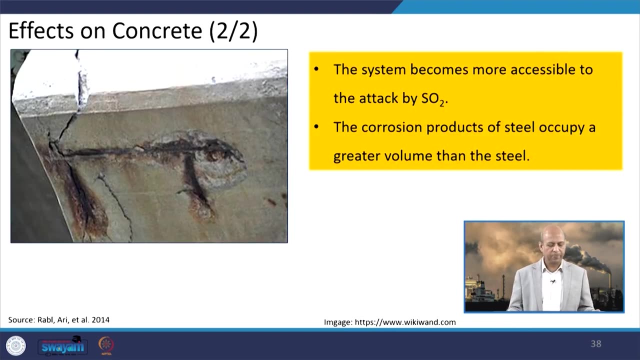 this is about the reinforced concrete. So, like these, steel rods, iron rods etc are there, so they are damaged by acid rain and rust happens and then volume increases, so further cracks developed in concrete and then concrete damage also happens. 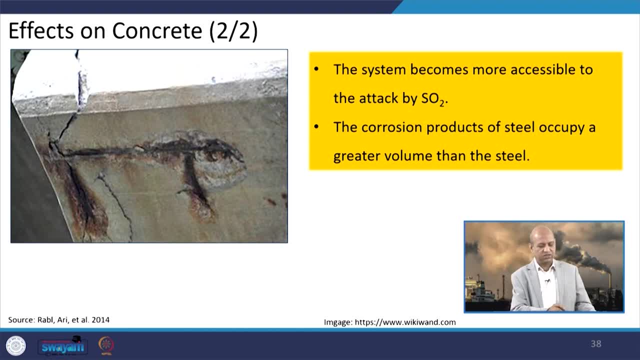 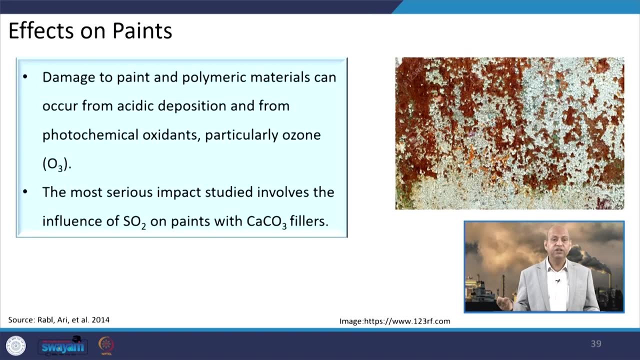 Well, when we talk about this kind of gaps, so you can see this corrosion starts and then damage continues. and on paints also, there are paints which can be damaged by like ozone, because it is very oxidizing, highly oxidizing gas, as you know. 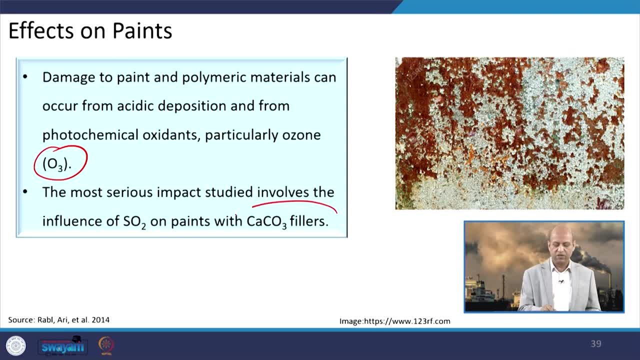 So because of these, and then there is presence of certain calcium carbonate fillers in the paint, So that can get affected by SO2 also. but ozone takes part initially and then the damage continues and it progresses quite high in longer term. So these kinds of things may be seen when paint is there but it is damaged by polluted 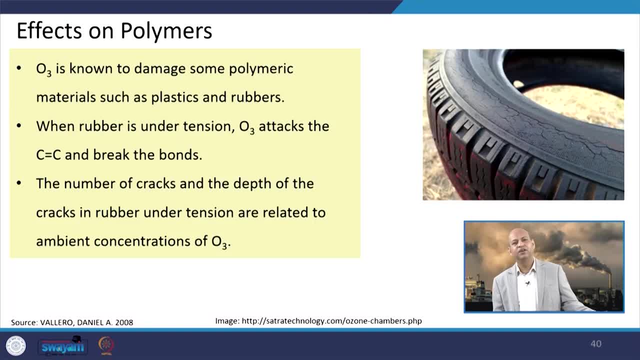 environment. When we see effects on the polymers like rubber or plastic those kinds of things, so they are badly affected by ozone because of this oxidizing nature. So you can see here cracks. These cracks are developed by ozone. So if ozone is very high in concentration in air, so there your tires will be damaged. 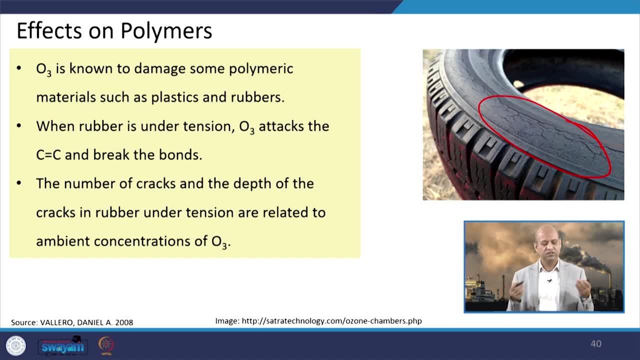 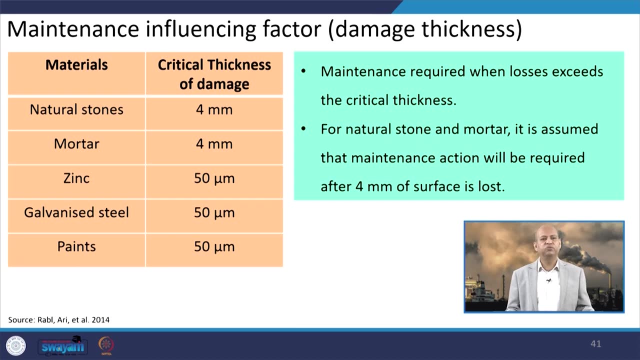 very quickly. So the economic effect is there. there are many other things And the number of cracks and depth of the cracks in rubber. it further goes depending upon the ambient air concentration and the usage of the tires. When we want to analyze the maintenance influencing factors, 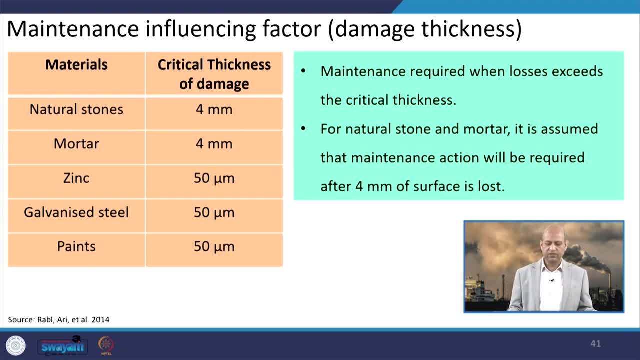 So you can see like natural stone if 4 mm is there. these are the critical thickness. basically Mortar 4 mm, zinc 50 micrometer, only galvanized steel 50 micrometer. paint 50 micrometer. This much of thickness, damage is there, then it is critical. 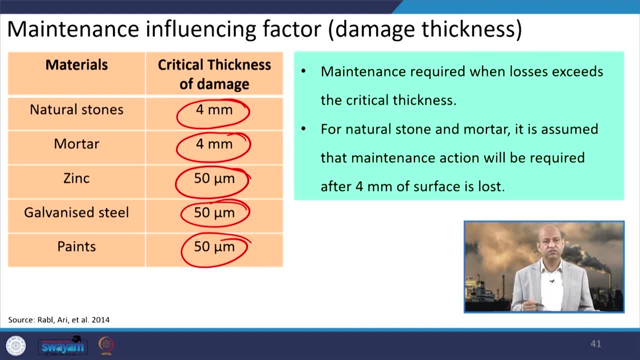 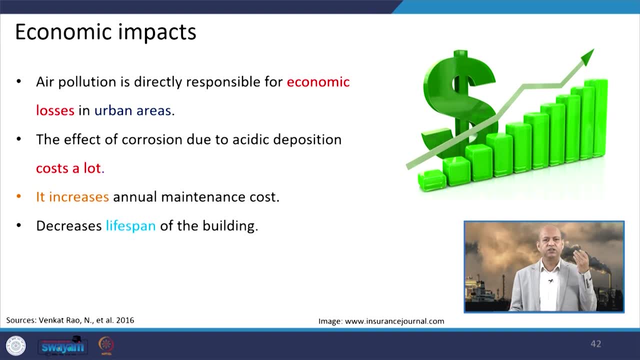 And one should go for some remedial measure, otherwise it will be highly damaged after some time. Then economic impacts. So you can see that Economic impacts are there, because when buildings are affected then we have to repair them and its age also reduces. structural components are also get damaged. 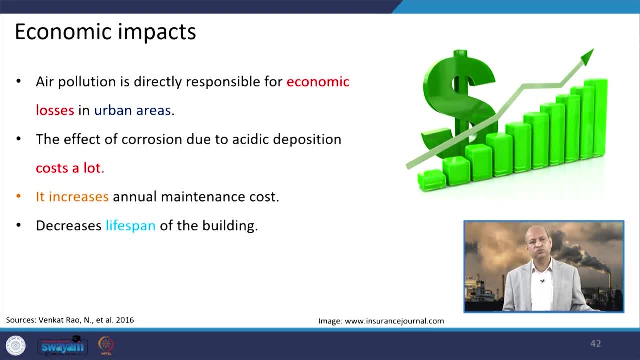 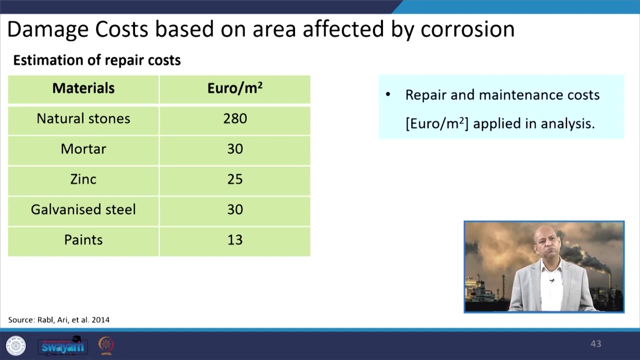 So economic impacts are there and the maintenance cost is also increased and lifespan of building is decreased. So economic impacts is severe if you do not care, if you do not deal with the air pollutants, cleaning from the environment, from the atmosphere, And the damage cost can be calculated, estimated. 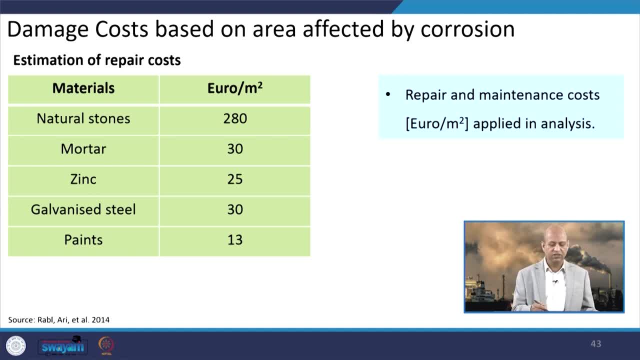 So you can see that. Okay, So you can see that the repair cost can be calculated by this kind of study. they have given this table that natural stones and the mortar zinc, etc. how much area of that is affected. depending upon the affected area, this repair cost can be estimated. 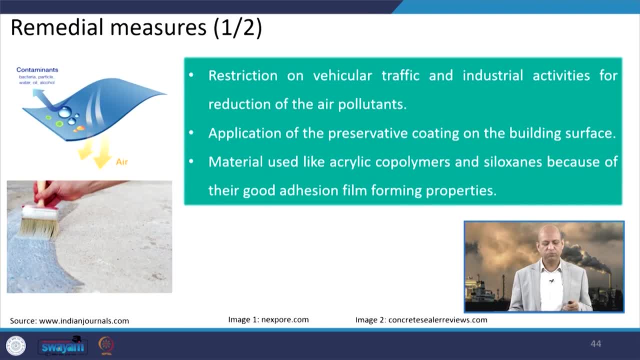 So that is used for estimation of the cost of damage because of air pollutants and corrosion. So remedial measures there may be, like coating. there are certain coating which bifurcates, which is kind of wall in between, very thin wall, so that this attack of the sulphur dioxide 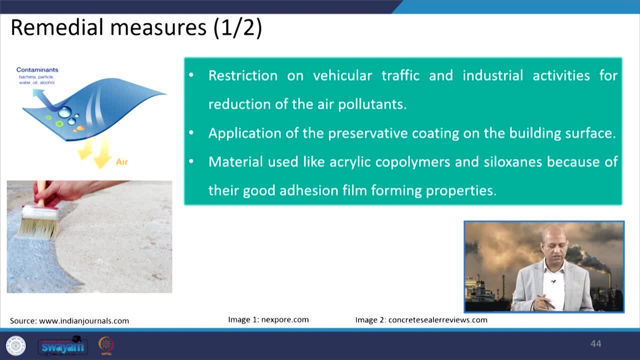 or acidic environment does not happen so quickly. Even you might have seen like nowadays, when you go to the car garage, they say that please get it painted by some coating the lower surfaces so that the rust does not happen. corrosion does not happen. 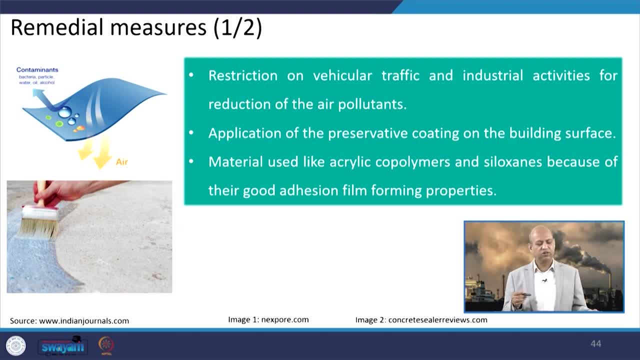 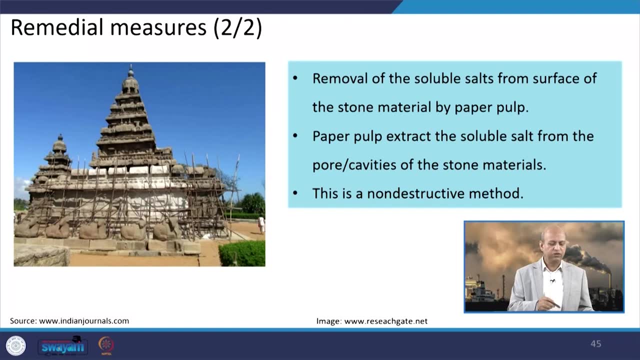 So those kinds of coating materials are there which can be used for remedial measures or to repair, So to reduce the ill effects or negative impacts of corrosion, etc. When we talk about building materials, stone related building materials, then there are: 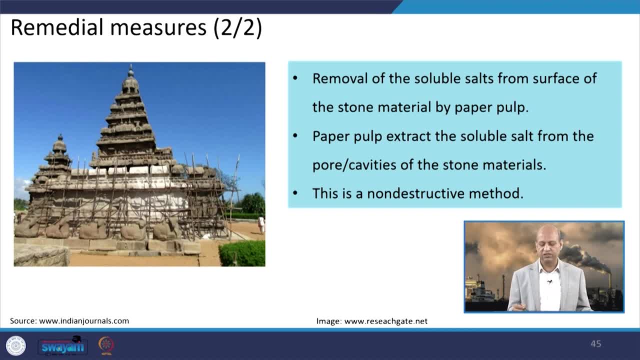 other ways to go for remedial measures, like paper pulp, which is used for this soluble salts removal. so this paper pulp related treatment can be done and this is a kind of non-destructive method. so it is a good way of removing those kind of material which was 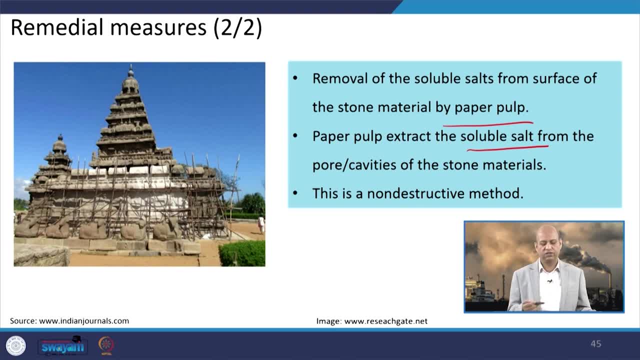 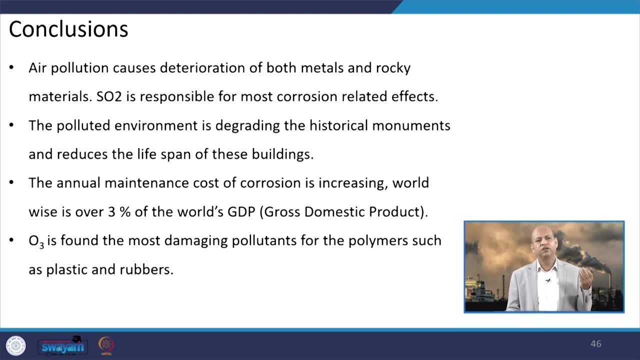 because of crust, because of those air pollutants damage. So in conclusion, we can say that air pollution causes several, not only the health effects but these effects on the buildings. they can cause deterioration, both the metals as well as the rocky material, and sulphur dioxide basically is major cause of corrosion related. 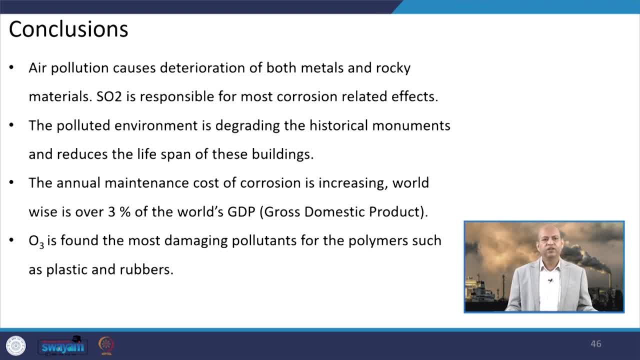 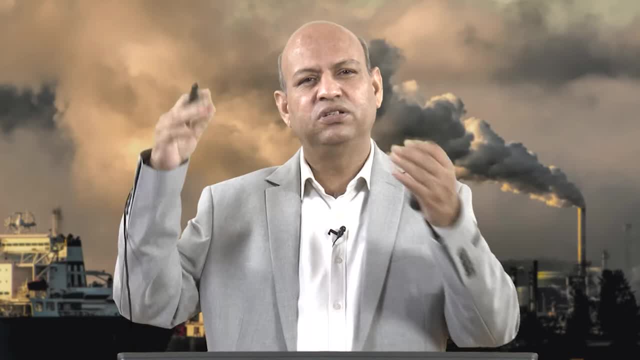 effects on the building materials and structural components, And the polluted environment is degrading the historical monuments you might have seen. whenever you visit some monuments, there may be some damage, so the damage may be related to weather as well as related to pollution. 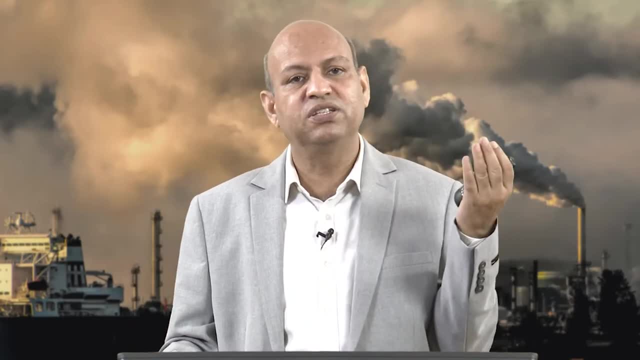 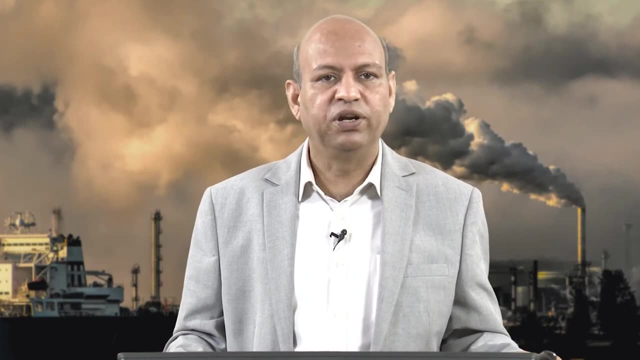 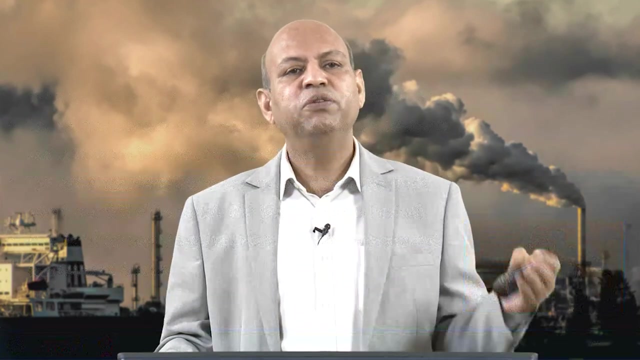 So our monuments have. they are very precious. we should protect them. so reduction of air pollution really contribute in protecting our historical monuments and it can increase its life span. otherwise the life span of these buildings will be decreased, Thank you. And the annual maintenance cost of corrosion is increasing worldwide over 3 percent of. 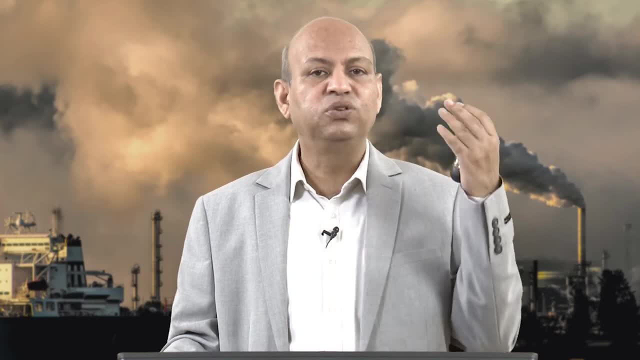 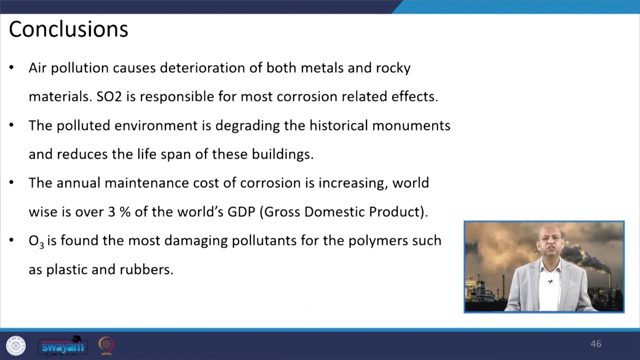 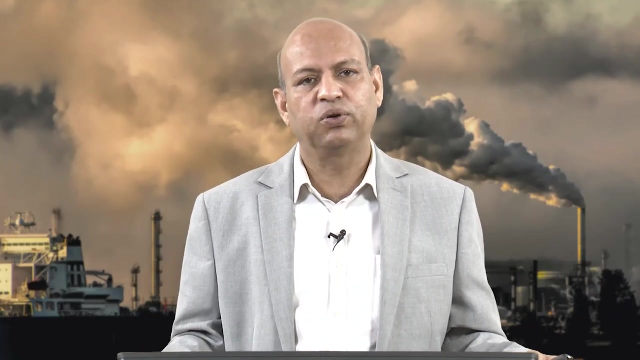 the world's GDP because of this pollution. so if we reduce the pollution, we can reduce this maintenance related cost also. And ozone has been found the most damaging pollutant for the polymer such as plastics and rubbers. so again, the property related protection. when we talk about then the reduction,